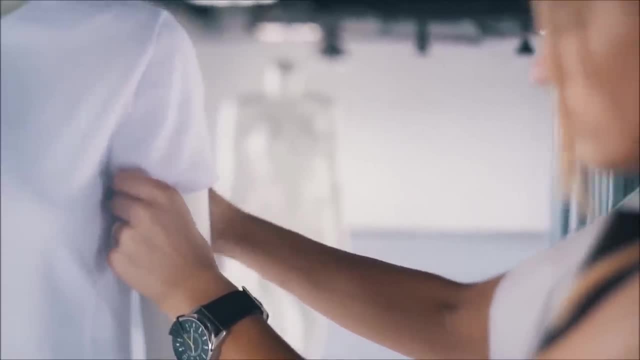 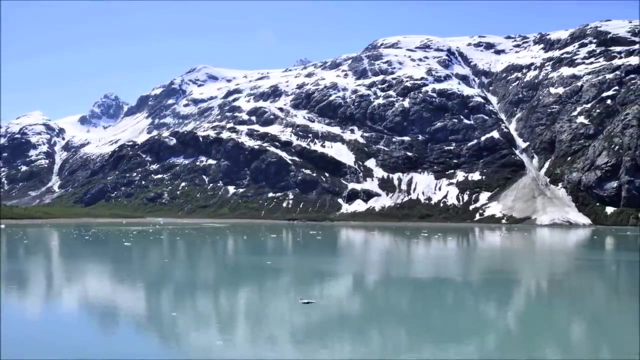 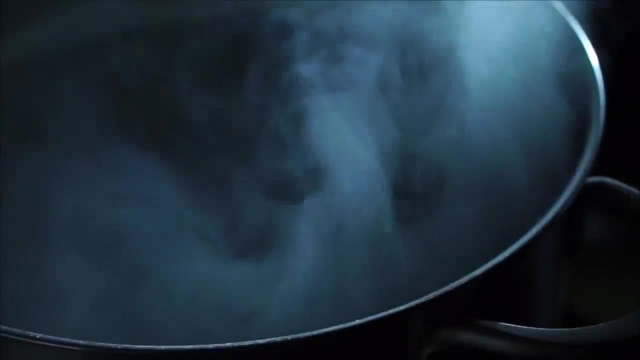 made of the same substance as the original cloth, just in a new form. Another type of physical change involves changing states of matter, and water is a great example of this. Ice melts and becomes water, and water evaporates to become steam. but no matter its form, the 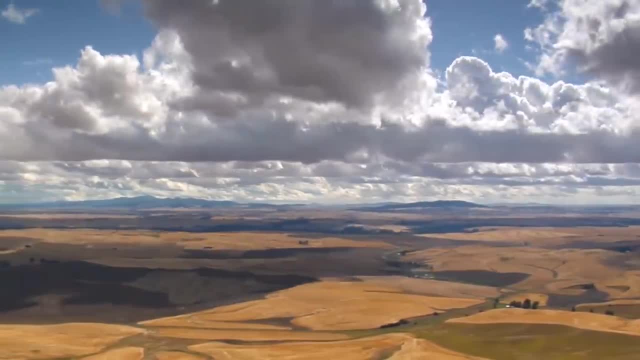 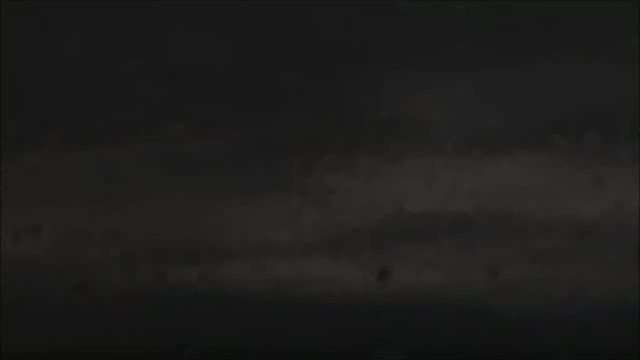 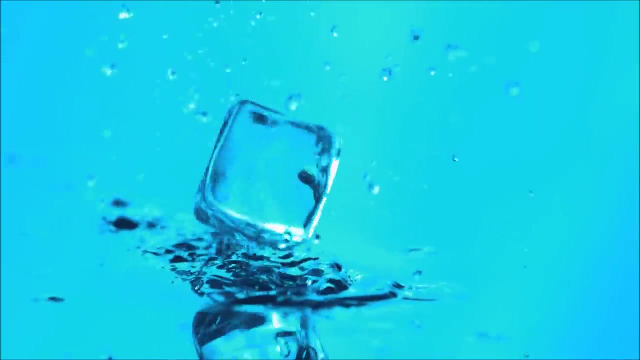 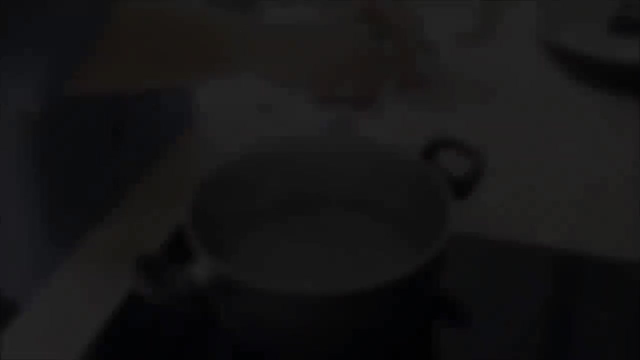 water is still water. One way we can tell this is a physical change is that the change can be undone. Water vapor can condense back into liquid water and liquid water can be frozen back into ice without changing to a different substance. In fact, many physical changes can be undone. For example, we know that dissolving sugar 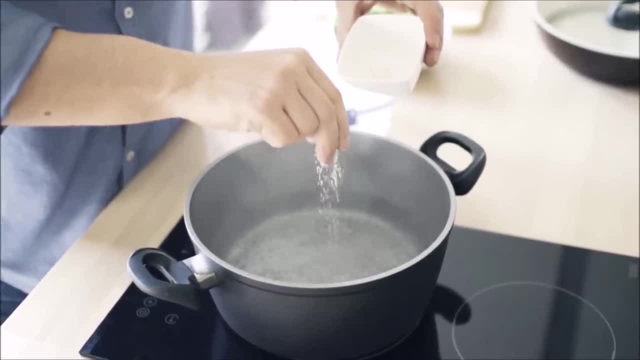 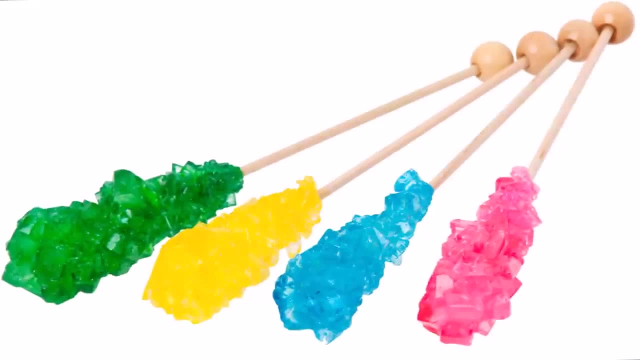 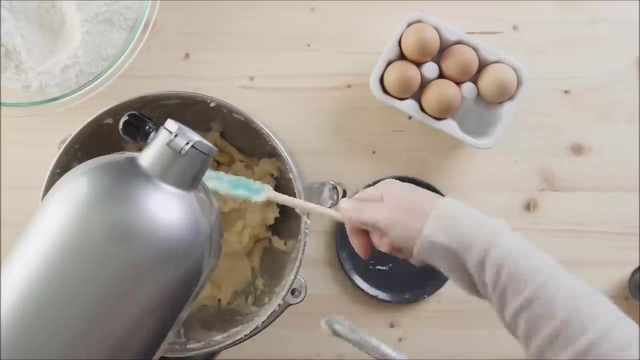 into water is a physical change because even though the sugar and the water are mixed together, they do not combine and create a new substance. They are still just sugar and water and they can be separated from each other. Not all mixtures are as simple to separate as sugar and water. When you mix butter, sugar 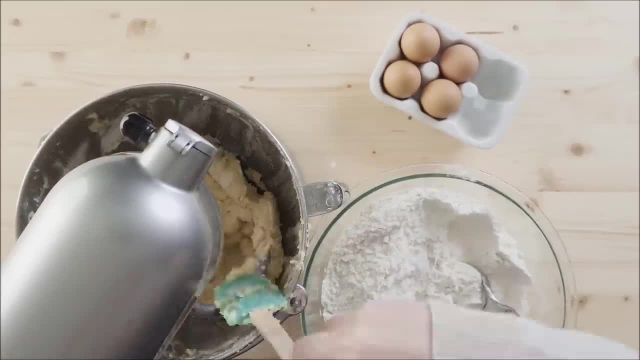 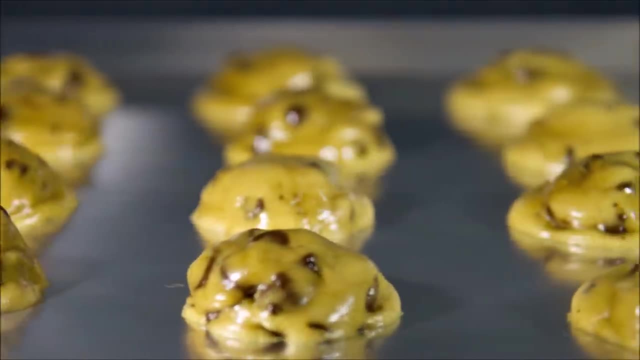 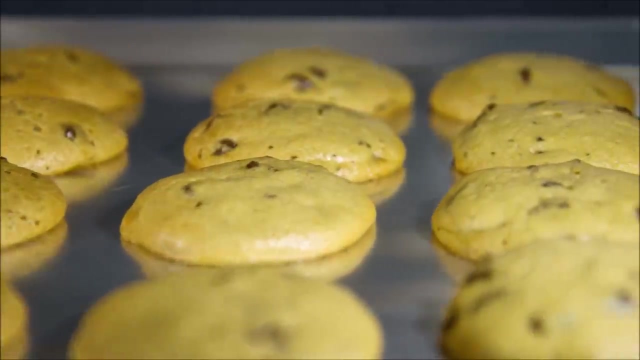 flour and eggs. there is not a practical way to separate them again, but it is still only a physical change. The chemical change occurs when you put your mixture in the oven and add heat. Baking has many of the indications of a chemical change. 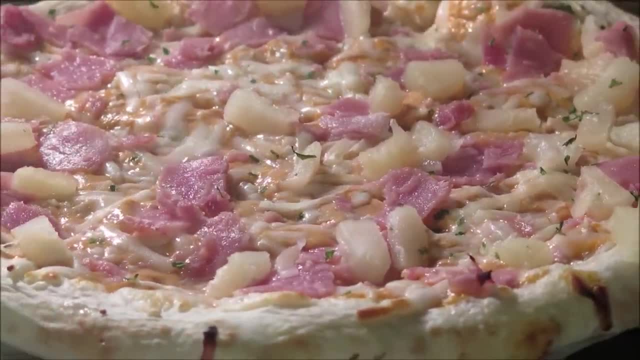 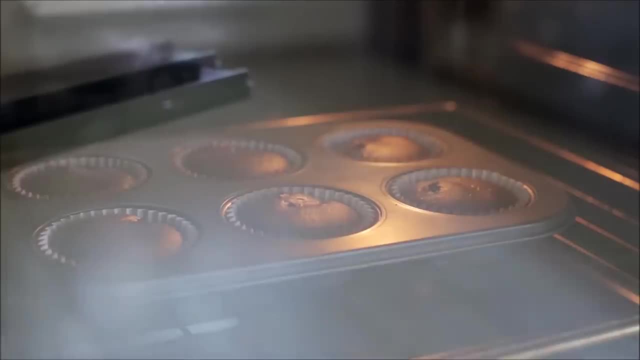 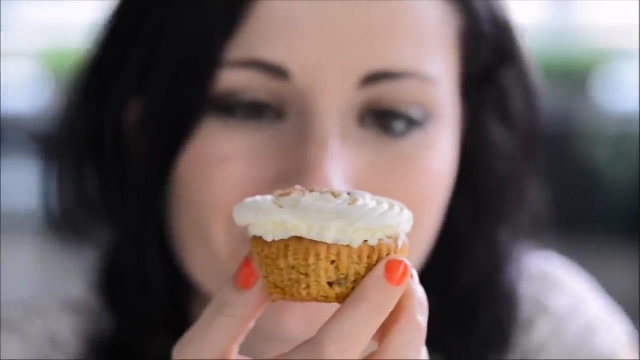 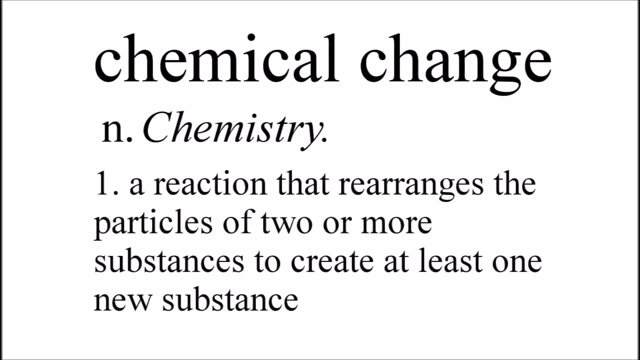 The mixture in the oven absorbs heat. It also changes color and produces an odor. Gases are released, which is what helps the baked goods to rise. Finally, this change cannot be undone. You can't unbake a cake. Chemical changes occur when the particles of two or more substances are rearranged to. 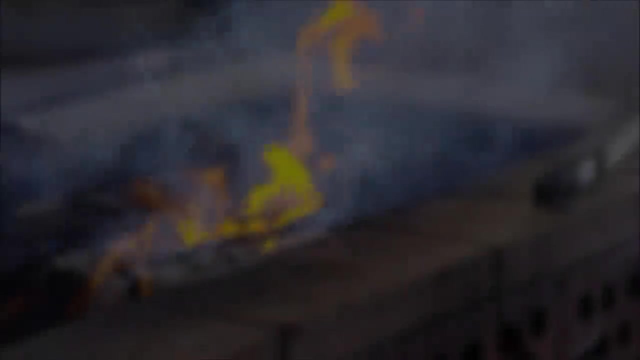 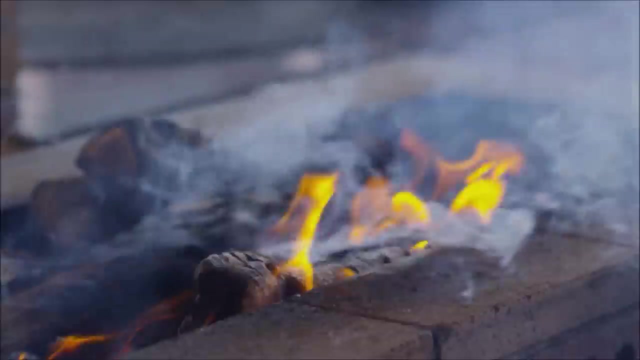 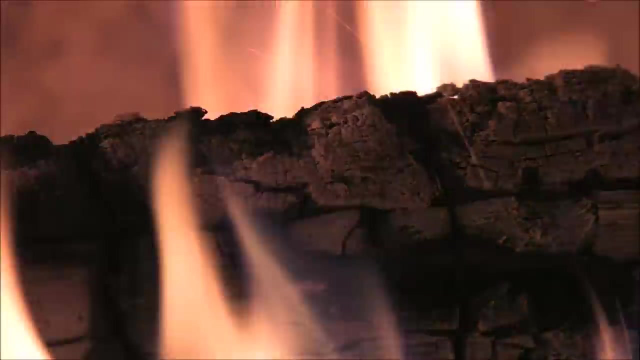 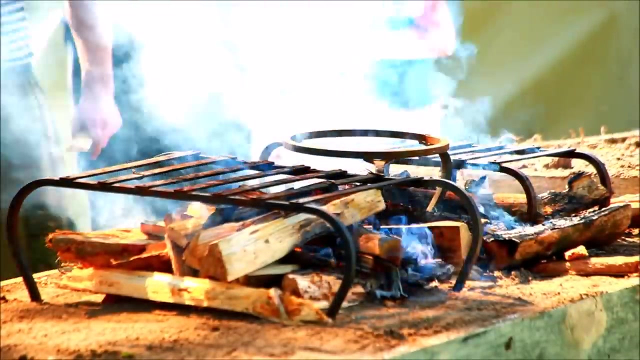 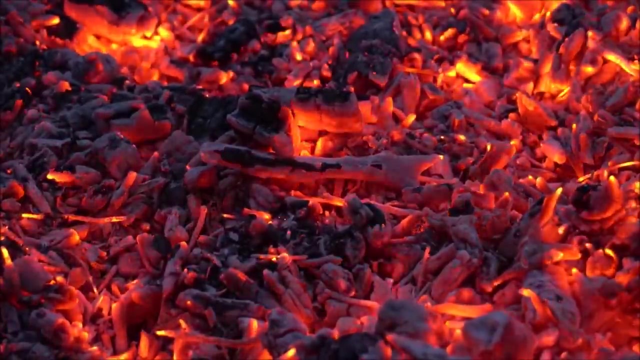 form a new substance. For example, when you burn wood, the wood is transformed into a new substance- ash. Just like in baking. this change cannot be undone. Also like cookies, the wood changes color, releases gases and produces an odor. Unlike in baking, this chemical change releases heat and gives off light. Chemical changes occur when the particles of two or more substances are rearranged to form a new substance: Ash-. In baking, this chemical change cannot be undone. For example, in cooking the wood changes color, releases gases, smoke and produces an odor. Unlike in baking, this chemical change releases heat and gives off light.